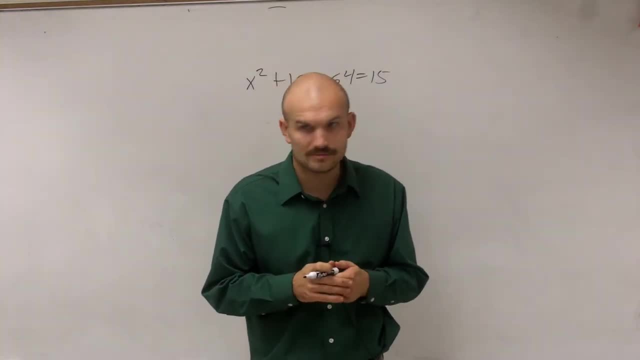 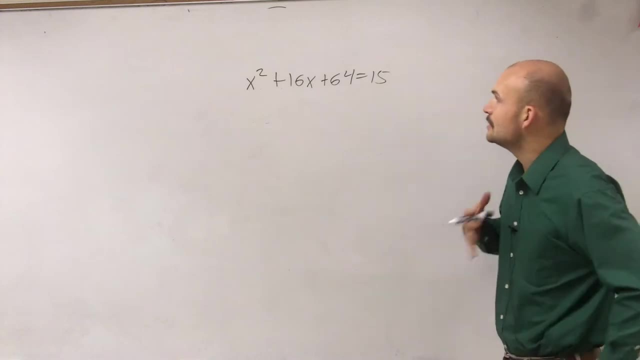 that's probably going to deal with taking the square root. Probably right, That square root method you kind of you know, thinking about that means you're probably going to have to take the square root. So what we're going to want to do is we're going to want. 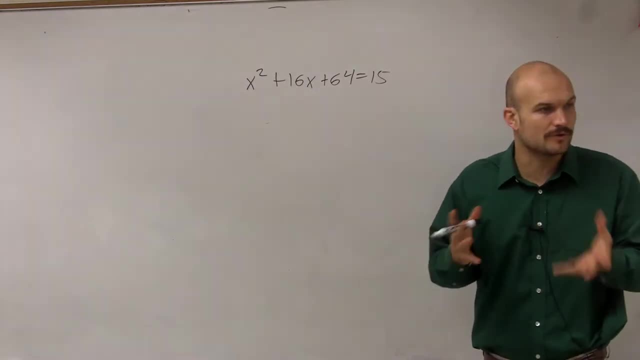 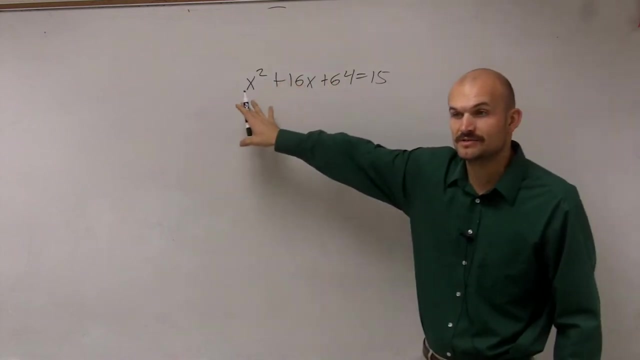 to see if we can get this to where we have a square root in there. Now, usually what we've always done, what I've told you guys to do, is, when you have a problem like this where we need to solve, we need to find the values of x. the first thing we always did was set. 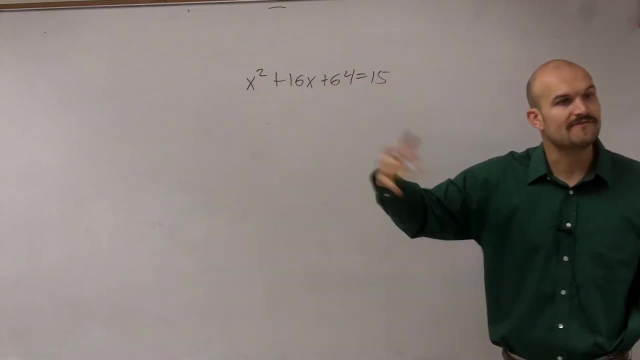 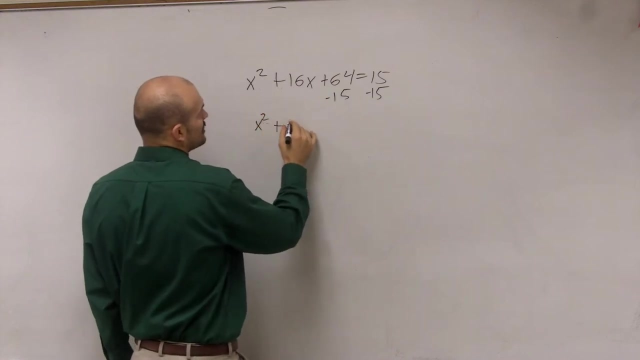 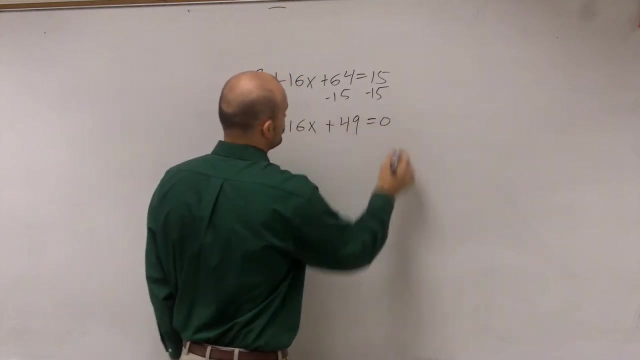 it equal to zero, Because when you set it equal to zero, you can factor it and use the zero product property. So if I was to do that, alright, I'd get x squared plus 16x plus, let's see 49.. Equals zero, Right? But then 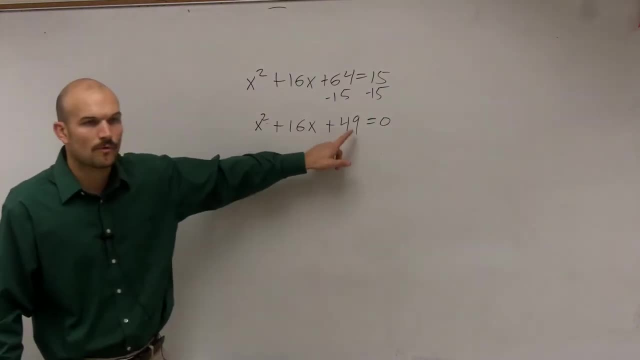 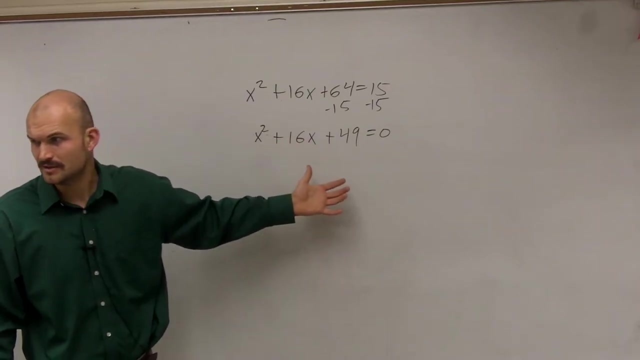 you need to determine is what two numbers multiply to give you 49, but add to give you 16.. And when you try to factor this, you realize that it's not factorable. Right, You can't factor this in what we've learned. So there's another thing that kind of comes up to this. 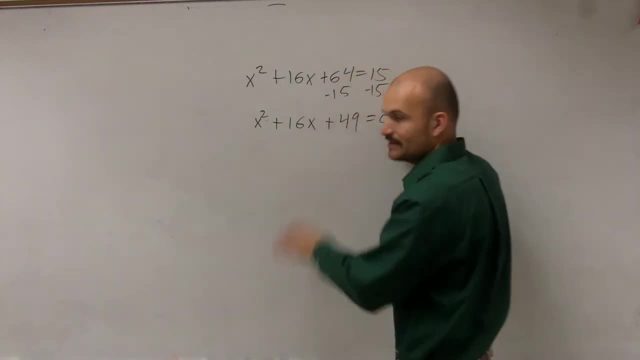 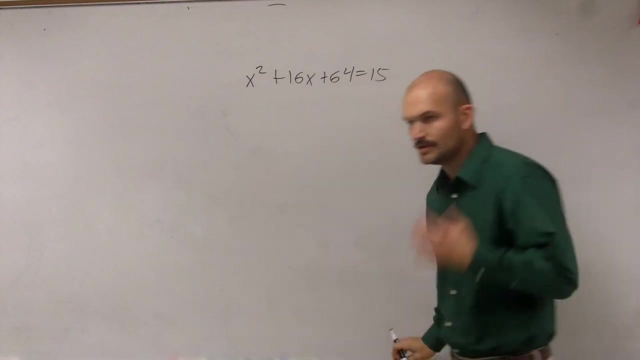 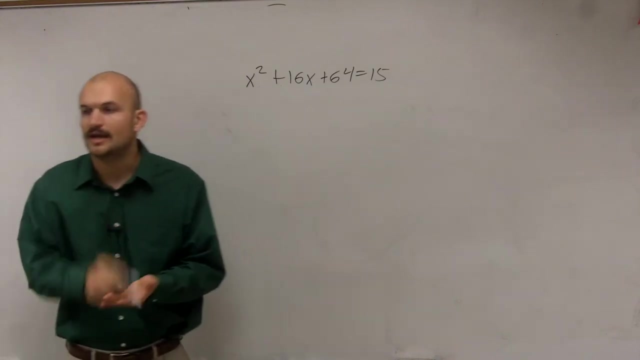 problem that you guys need to understand and look for. So this method is not going to work because we can't factor this expression to use the zero product property. But what I notice and you guys got to look for these, you got to look for your square numbers. You got 4, 9, 16,, 25,, 36, 49,, 64,, 81,, 100,, 121, 144,. 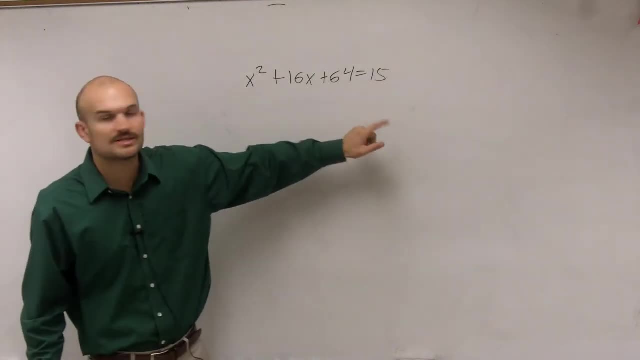 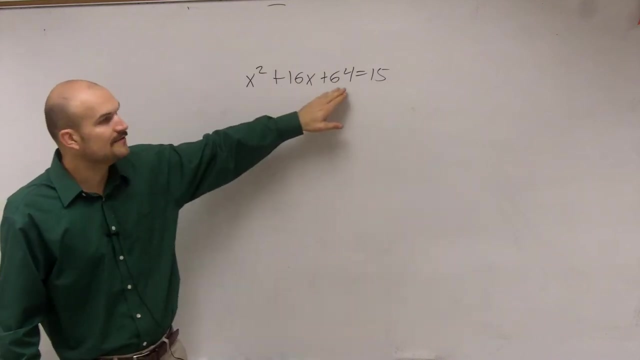 169, 196, 225.. What you need to notice is you look for those square numbers. If you see a square number, always look for either difference of two squares or see if you can write this as a perfect square: trinomial 64, that's a square number, Right If the square number that's 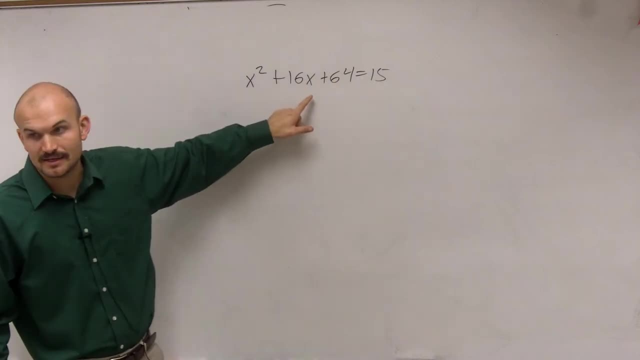 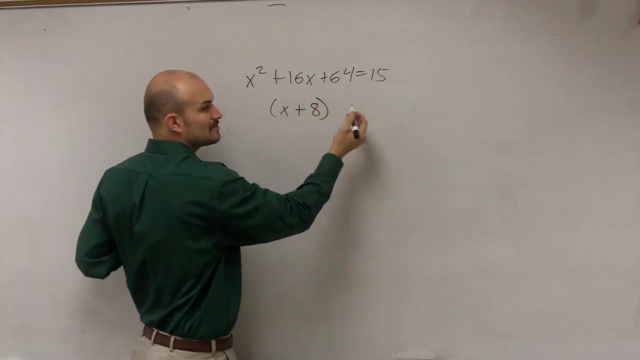 really 8 squared. Does 8 plus 8 give me 16?? Yeah, So I can factor this really quickly and just say: it's x plus 8 times x plus 8.. Right, Or I can just write x plus 8 squared.